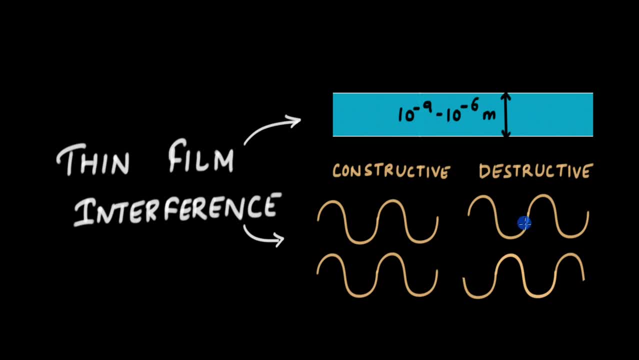 the drops line up with the peaks. this sort of situation leads to destructive interference. All right, now that we have some idea of what each of these words mean, let's bring back the soap bubble. So here it is. joke Alsonational. 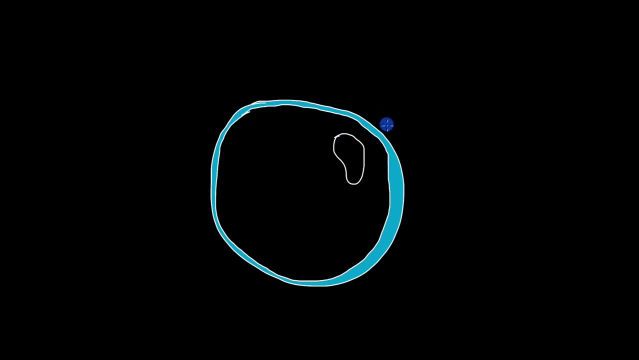 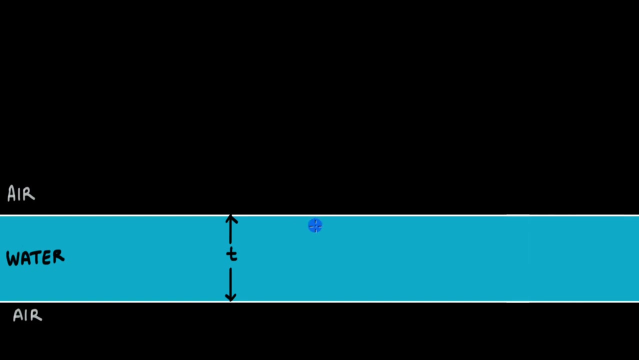 So here it is. Well, the wall, the wall ofí, well, the depopulated. it's just a thin film, that î of water. this is water that is between two layers of soap. now let's zoom. let's zoom into this. so we have zoomed right into one small, tiny, microscopic section of the soap bubble. 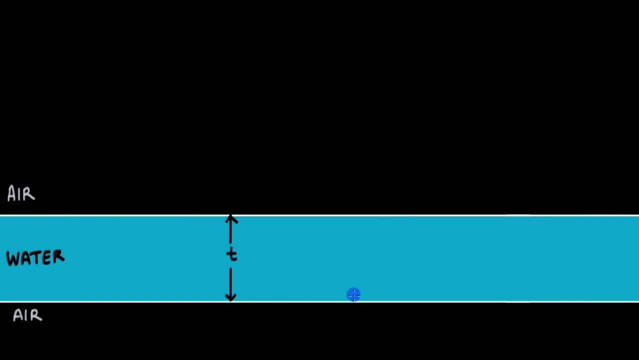 such that the such that the layers almost seem like straight lines. so this is the thin film. there's water in between these two white layers of soap, the white lines, the white layers of soap now light from the sun, which has colors of different wavelengths, so red has the longest. 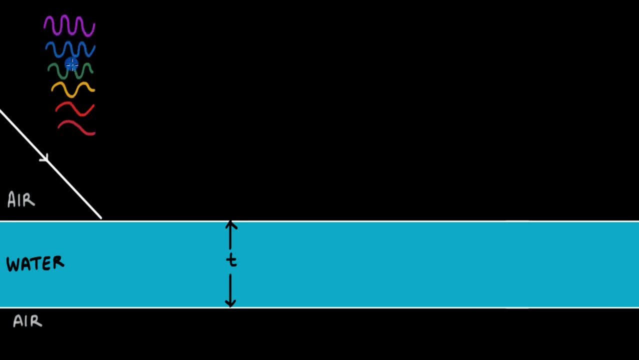 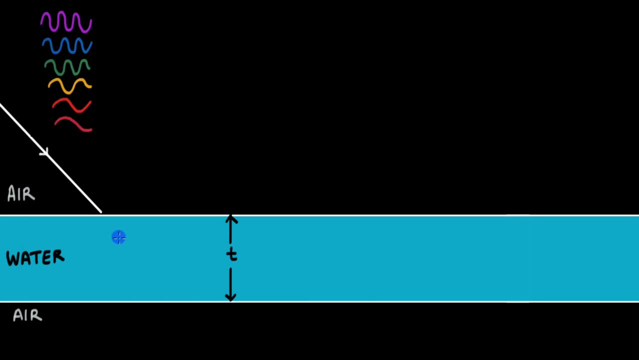 wavelength and violet has the shortest wavelength. there might be a color missing over here. i think that's blue. anyway, this is light, is incident on the top surface of the thin film and because there is a change in the medium, it undergoes refraction and then coming out of the bottom surface of the 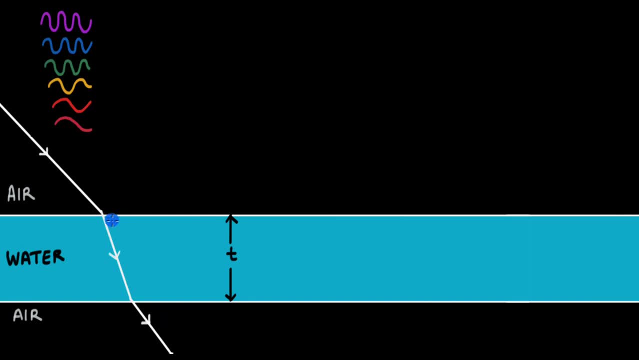 film. it gets refracted again but turns out some of the light reflects back from the first surface, some of the light is refracted and some of the light is reflected off the top surface and some of the light is reflected. some of the light is reflected from the bottom surface. 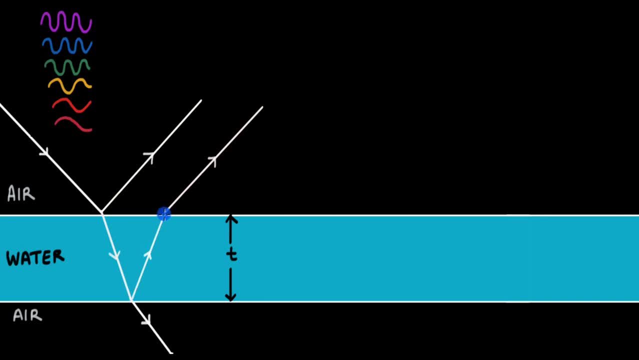 after undergoing reflection. at this point it undergoes refraction and it comes out parallel to the first ray. now the key here is that wave number one, wave number one and wave number two. they travel different amount of distances. the light wave reflected from the second ray of light- i can clearly see this from the hyperscale data- one is when it Fernando. 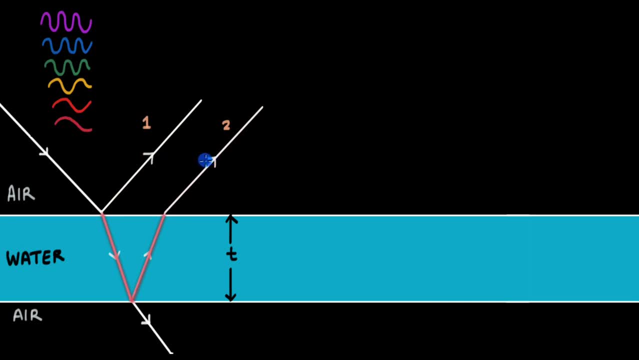 now about the power or weight of the light child is because it travels this much extra distance. so there is a path difference between these two waves, between waves one and two. now, these two waves, one and two, they are quite close to each other so they can meet an overlap, they can. 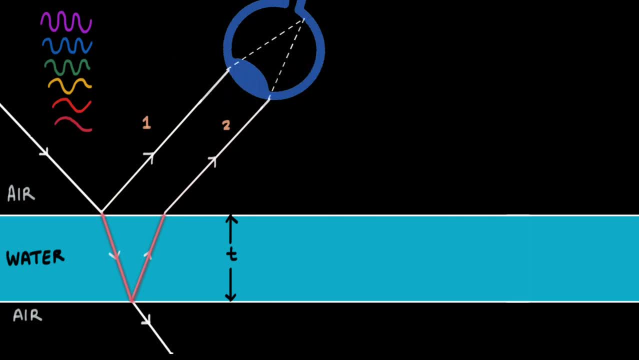 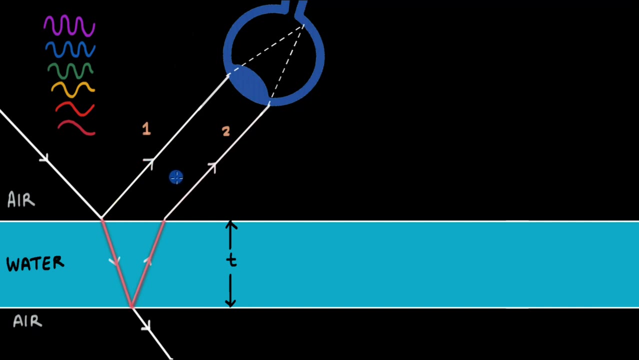 interfere and our eye that can be, that can be on the top. this is the entire eyeball. the eye can lead to either constructive or destructive interference, depending on whatever this path difference is now, as there is a part difference, waves one and two could either be in phase or 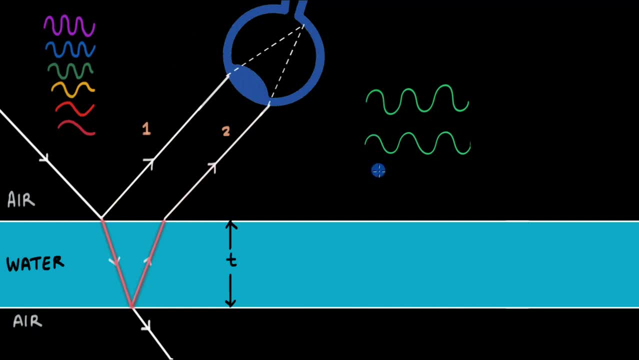 out of phase. if they are in phase, then their peaks would match with the peaks and troughs would match with the troughs. in this case they will constructively interfere and we will see that color. so if the green light constructively interferes, we will see a green color film. 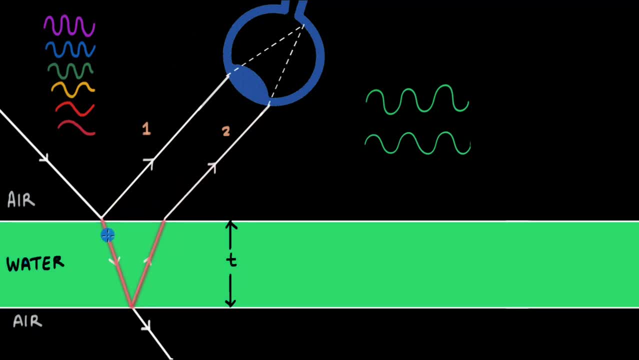 but there could also be a possibility that, as a result of this part difference, waves one and two are out of phase and the peaks are matching with the troughs and the troughs with the peaks. in this case the waves will destructively interfere and we will not see that color. 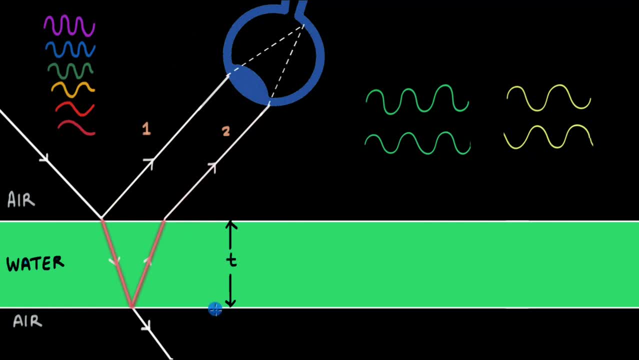 in that section of the soap bubble, this thickness of the soap film. it determines the part difference and if you change the thickness you can change the part difference which could lead to different colors interfering constructively and destructively. that is one factor on which, whether the lights are interfering constructively or destructively. 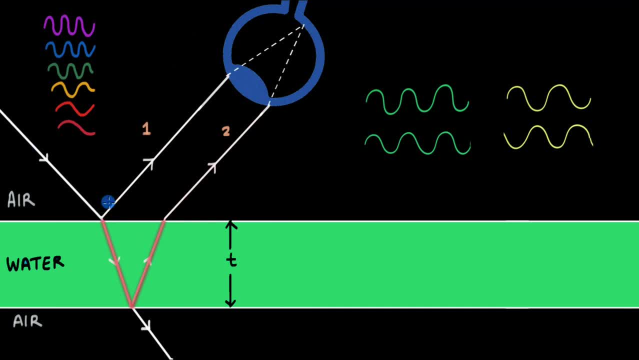 depend upon. the second is also: you could imagine the angle of this, the angle of this incident light. if this angle changes, the part difference will also change. if this incident angle was more, that is, if the, if the incidental ray of light came from this direction, then the part difference 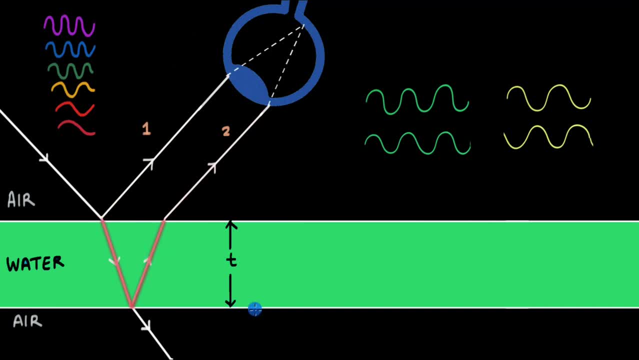 would also be more in that case, as the light will get refracted and then go back, so it will be traveling more, more distance, and maybe because of the fact that the lights are interfering constructively on different sides of the soap mom orperzie, because of that part difference we might. 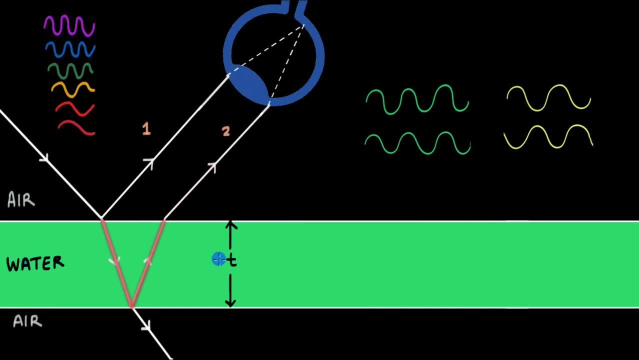 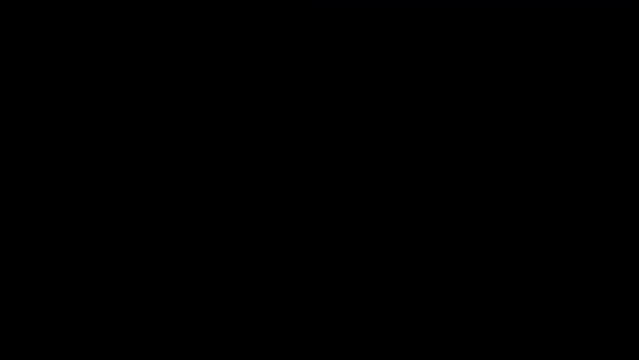 see constructive interference of some different color, maybe not green. so the angle of incidence and the thickness of the soap film can determine which light will interfere constructively and destructively. and this thickness, it, varies or changes all over the soap bubble. so different wavelengths of light are interfering constructively or destructively at different parts of the bubble. 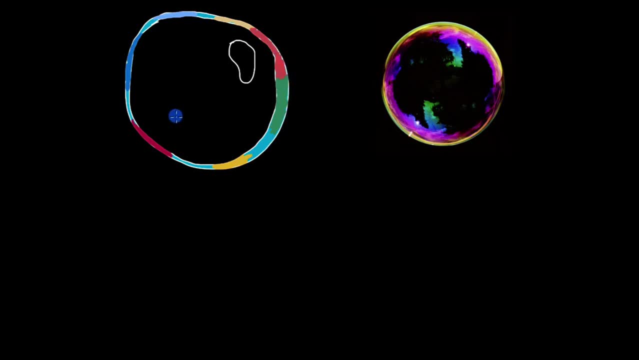 see, we see different colors in different areas of the bubble, and that's why we see these really cool rainbow colors. what about? what about the butterfly? though? now, the blue color here is not due to a pigment color of the wings. in fact, the pigment color of the wings of a blue morpho. 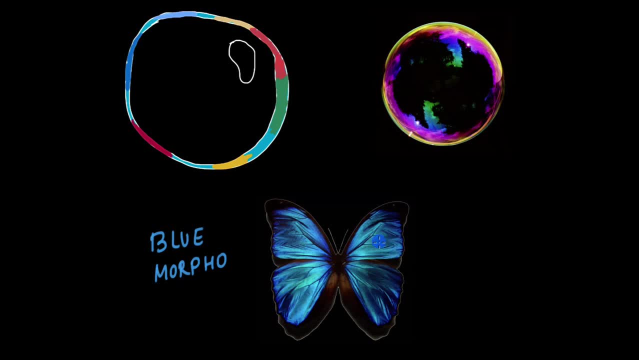 butterfly is brown. it's not blue, but the color is due to due to thin film interference, but more specifically, it is due to the structure of the wings. if we zoom into the wings, the wings of the butterfly have these tiny, microscopic structures with air gaps in between, and they act as multi-layer. 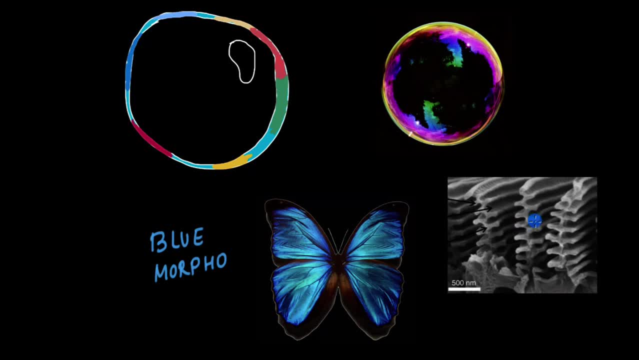 thin films. these films are just the right thickness for the blue wavelength of light to constructively interfere and for all almost every other wavelength of light to destructively interfere. and that's why we see this, you, we see this vibrant blue color on this butterfly. let's talk about why we don't see such patterns with a water drop or a window pane. 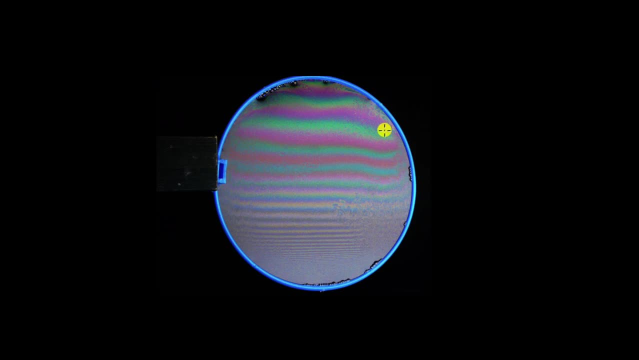 for this we take the situation of a vertical soap bubble, since, since this film is vertical, it is thinner at the top and thicker at the bottom due to gravity's pull. so the cross section of the film can somewhat look like this: thin at the top and it gradually gets thicker and thicker near the bottom. 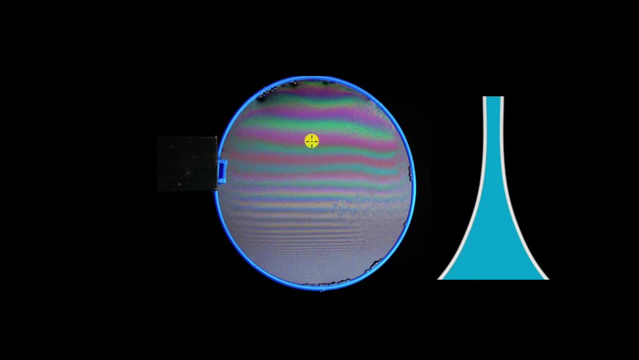 we see. we see that the fringe pattern is clear and distinct in this, in this section of the bubble, and as the thickness increases, the fringes start getting close to each other until we are barely able to separate them and we end up seeing white at the bottom or 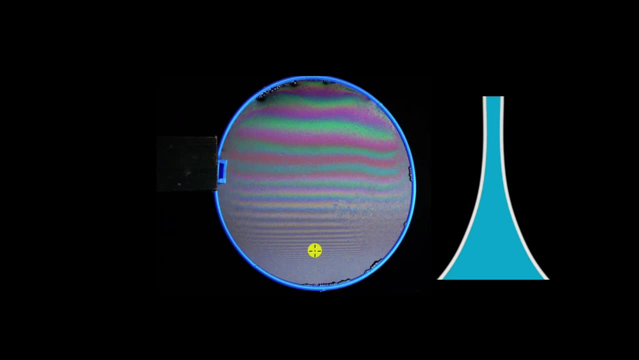 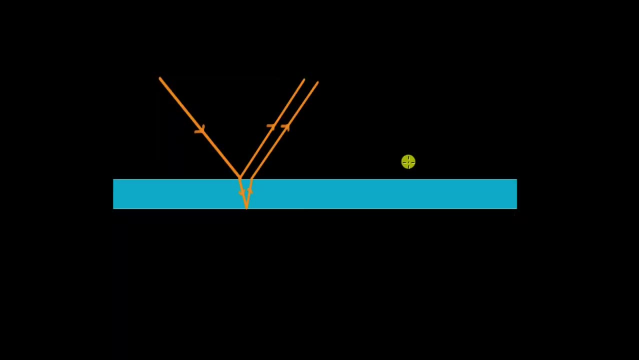 washed out, white more or less. why does this happen? let's, let's look at the thin film again now. this yellow light can interfere constructively, but to get a different color we can change the thickness or the angle. we are not changing the thickness right now. let's, let's just change the. 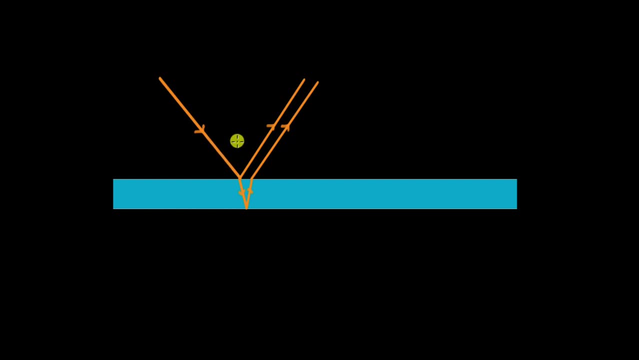 angle and see what happens if we, if we change the incident angle. if we change this angle slightly, then the ray of light could be coming from here and it will undergo refraction and then reflection. but but there won't be much change in the part difference, right, because the thickness here is. 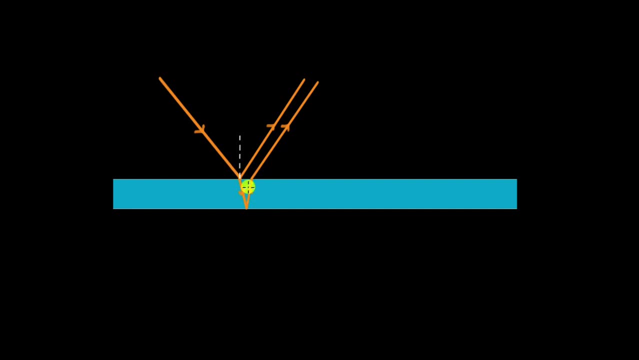 at the same order as the wavelengths of the light that are incident on it. so if we change the angle slightly, just slight change in the angle, we are giving some extra part difference for it to move through the film, but not enough for, let's say, a different color wavelength of light. 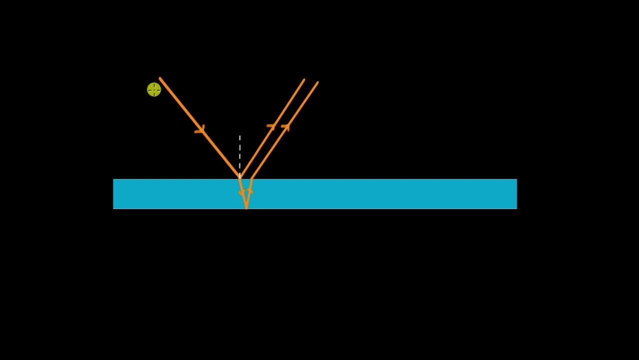 to interfere constructively on on slight change of the angle. we will still see yellow light, but maybe not as bright, though we will still see yellow light if we change the angle enough, maybe like this, so that now you see how much extra distance the light is traveling inside the film. 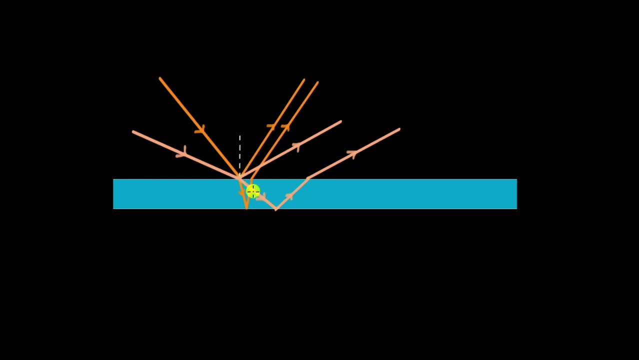 you're giving all this extra part difference. the total part difference would still remain as this total distance, but now it is traveling some more distance. there is some more part difference. there is an extra part difference. maybe we have changed it enough so that a new color with a different wavelength is now in phase due to the extra part difference. 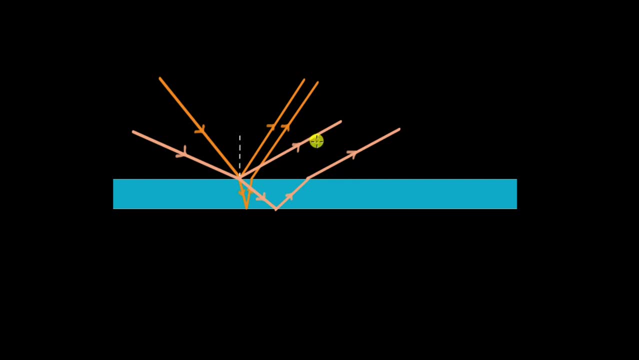 then we will start seeing that color. now we will start seeing orange color, and this tells us that the fringe patterns here will take some space for themselves. you need to change the angle enough so that you see a fringe pattern for a different color. therefore, in this section where the, where the film is relatively thinner, 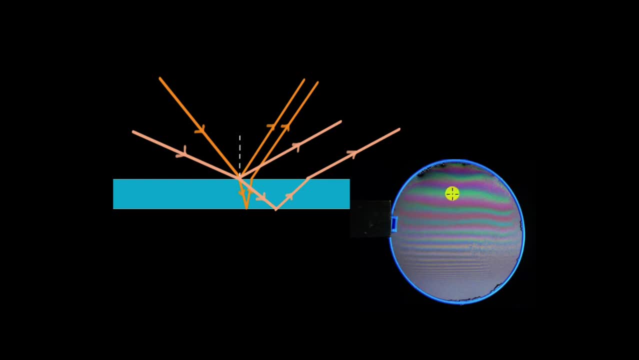 we. we can easily separate out the fringes. we can easily see where the green is ending, where the red is beginning, where the blue is ending, where the yellow is beginning. our eyes can make out where one color ends where the other begins. but when the thickness is increased, let's see what. 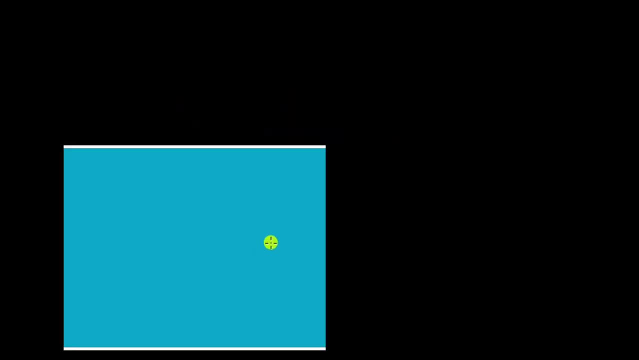 happens then. so here we have a really thick film. now maybe yellow light is interfering constructively to begin with, and we change the angle slightly. so again the the normal. here it is. now we are changing this angle, this incident angle, just slightly, just a slight change. and let's see what. 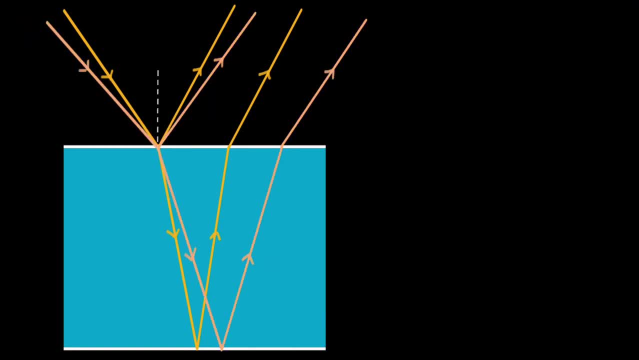 happens then? so maybe the new rays, the new rays might look like this. let me make this transparent slightly so that we can see this. all right, just a slight change in angle and see how much extra path difference we can. we can see that these two sides, these two sides are considerably larger than 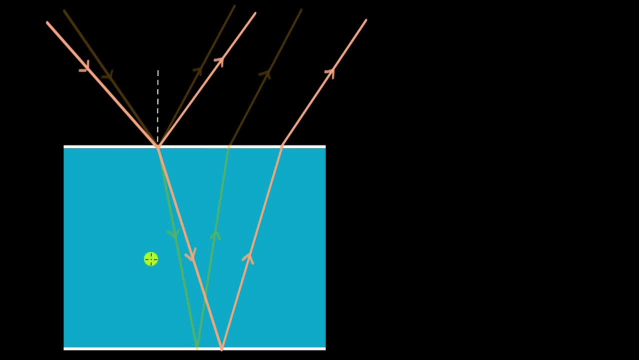 than these two sides. just a slight change in the angle and there is so much extra part difference. maybe one entire wavelength, who knows, could be two wavelengths, but the idea is that now the light has to travel much greater distance even with a very slight change in the angle. this amount of extra